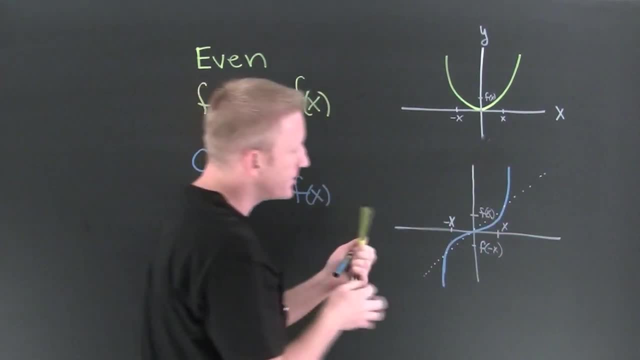 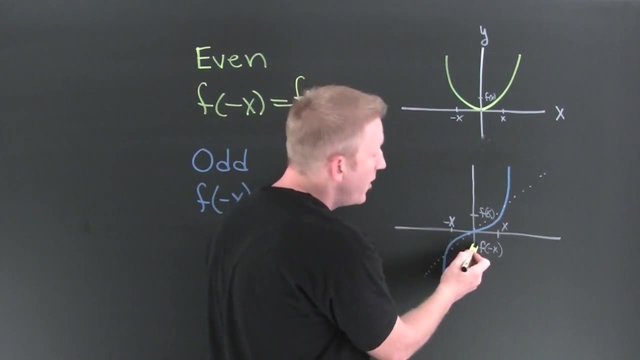 Yes, If I take a look at this man, f of x is right here, Yes, And then minus x is right here. What do you notice about these two? They're on opposite sides of that line, And that's what this says. 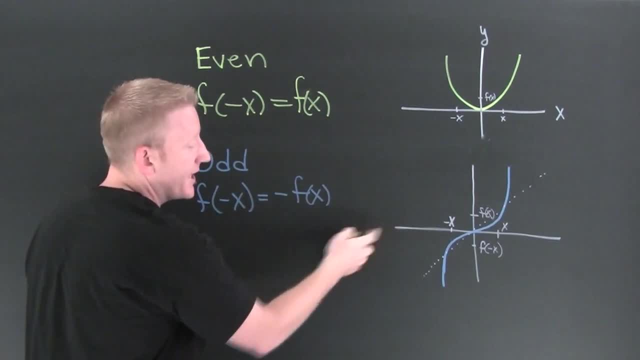 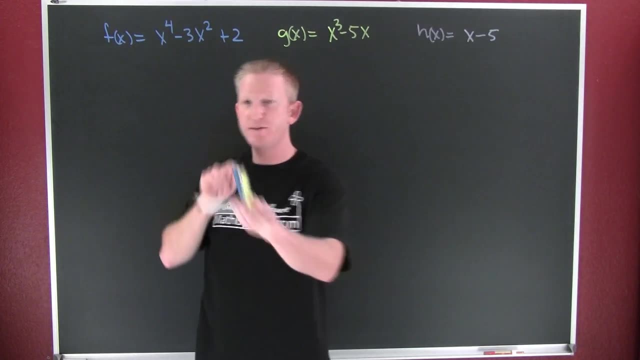 That these two guys are going to be on opposite sides of the x-axis. Okay, Why don't we get to some examples? Okay, So we're looking for these properties on up in here. What do I want to do? I'm going to check this thing thing. 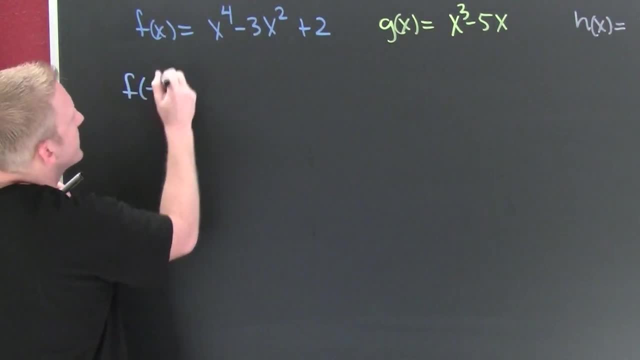 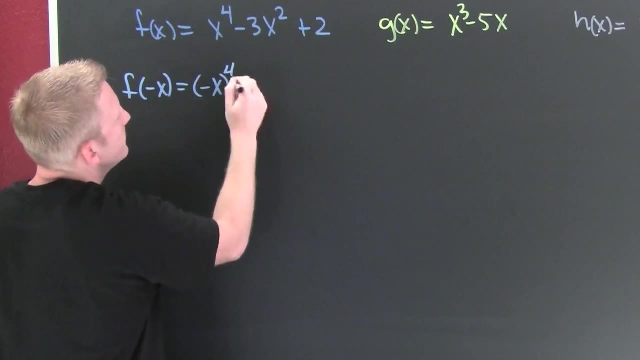 I want to take a look and I want to try to find f of minus x. What does that mean? Everywhere I see an x, I'm going to put a minus x and I urge you use parentheses. Okay, Minus three times a minus x squared plus- oh, wait for it, two. 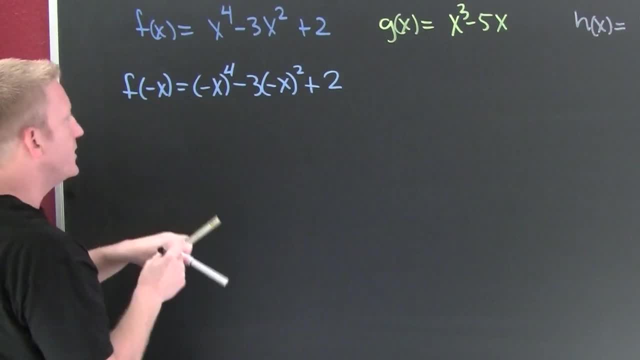 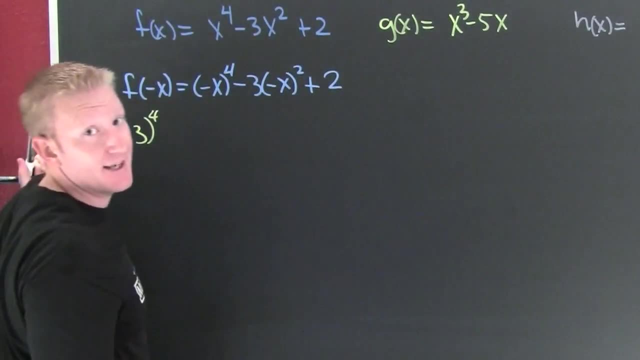 Oh, Let's take a look at this man. If I had had something like that, yes, If I had had minus three to the fourth, just saying right, You could see this as minus one times three to the fourth, which is the same as minus one to the fourth, three to the fourth. 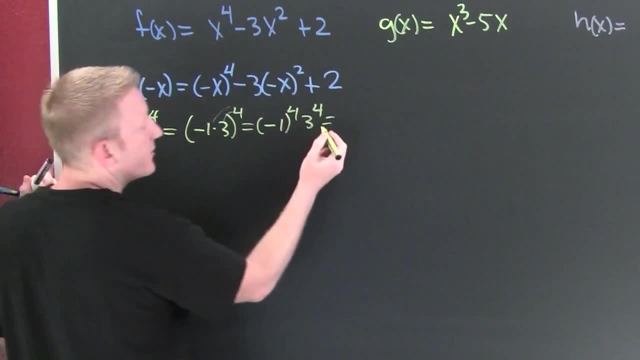 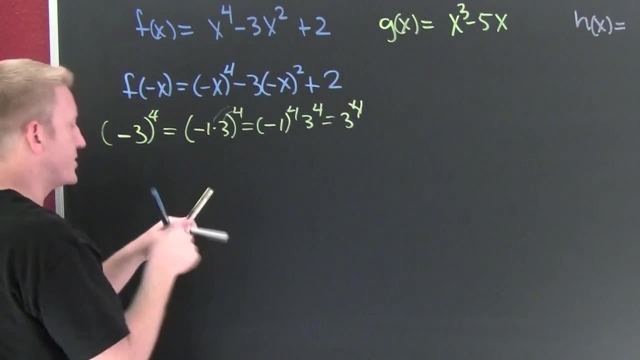 When you do this bam bam. So then, what's that? minus one to the fourth, It's one, And you end up with three to the fourth. Okay, What am I doing? I'm using that to justify this Rationale. 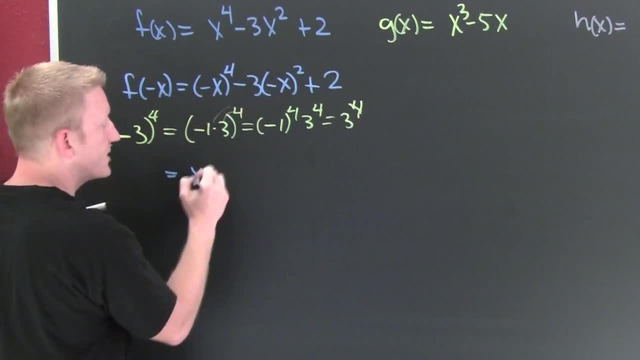 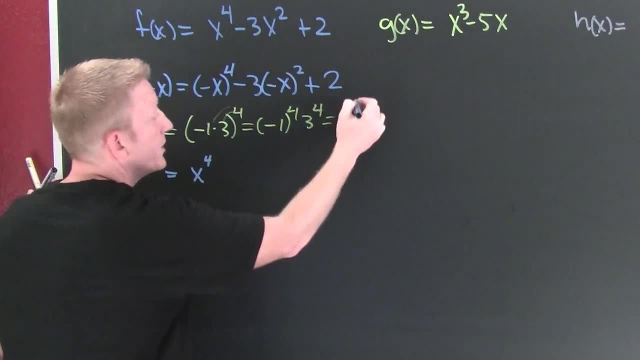 Mm-hmm. Minus x to the fourth is the same as x to the fourth. Yes, Why? Because the even power is going to- for lack of a better word- kill that minus sign. Mm-hmm. It's going to make it positive. 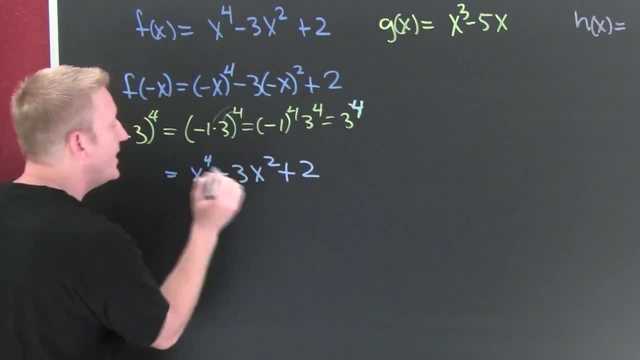 Minus three times x squared plus two. But what is that? That is f of x. So what do we have here? We have: f of minus x is equal to f of x. So what do you say? Dot, dot, dot. 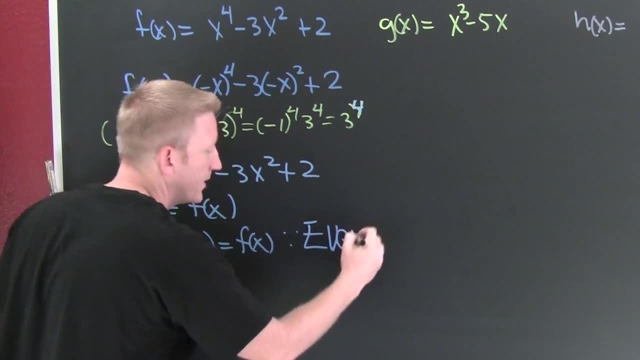 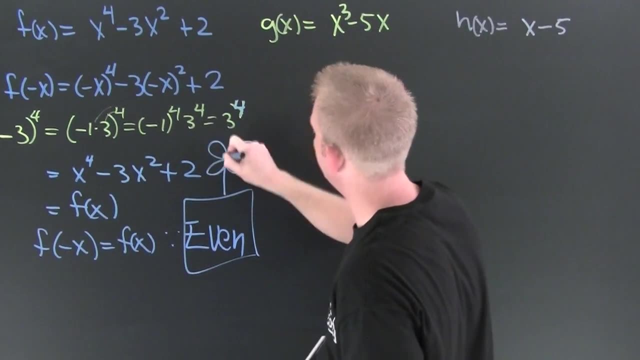 Even Okay, On up here. Ooh, Did you want boxes? Did you want flowers? Woof, woof, woof, Uh-huh, Up here I want to perform that same type test. Yes, I want to look for g of minus x. 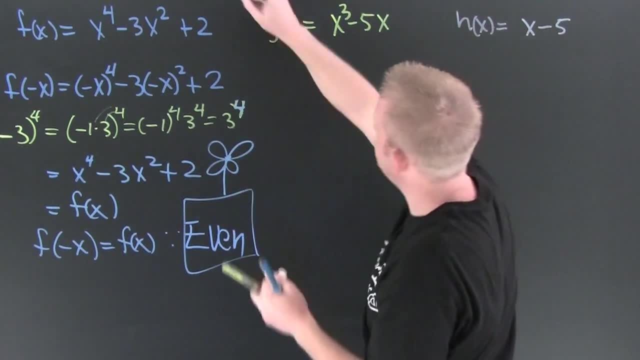 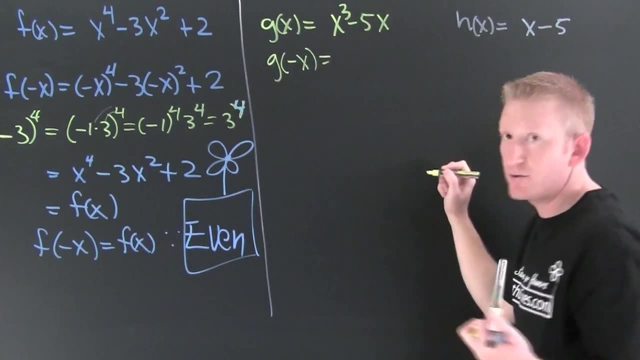 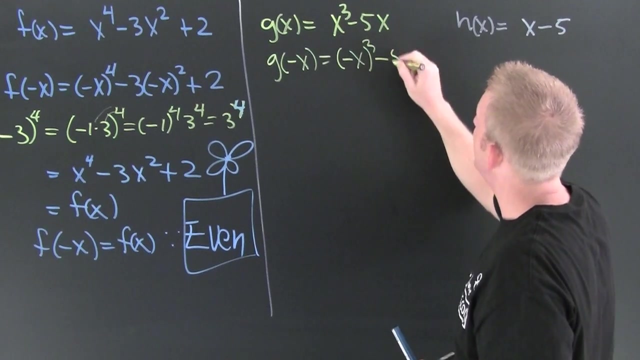 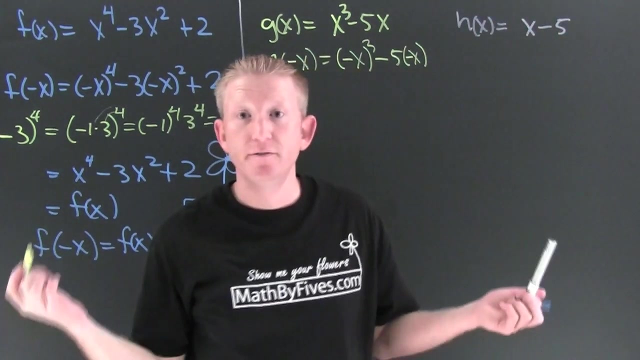 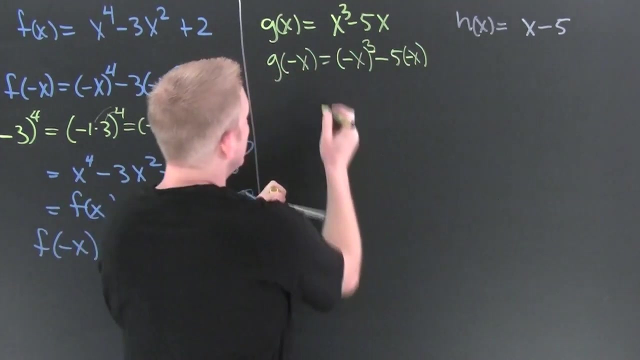 Then I go. when I throw that in there, this is minus x to the third, minus five to the fourth. Okay, Minus five times minus x, Okay. So take a look at this man. For the same reason, on the evens, the odd exponent is going to pass the negative out. 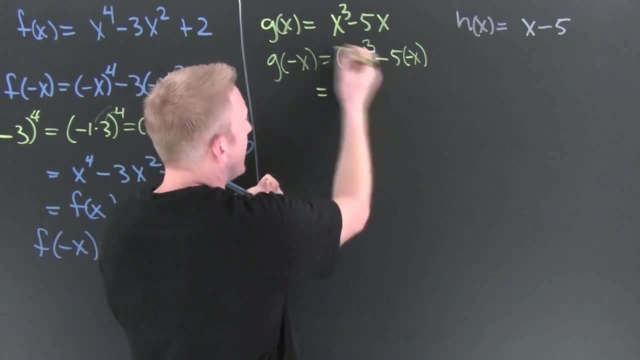 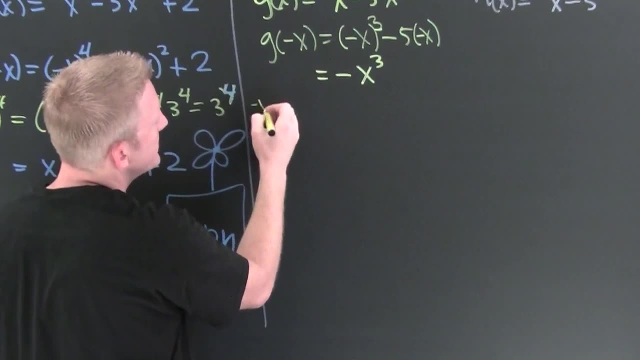 I want to pass out. Maybe you wanted to see it. No, Okay, I'm not. This is going to be minus x to the third. Why, Fine, I will. If you had minus x to the third. that's going to be minus x to the third. 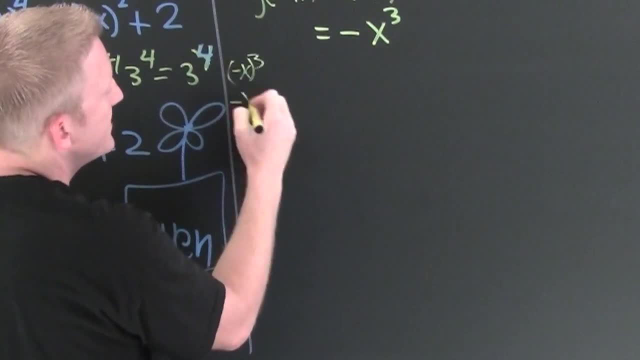 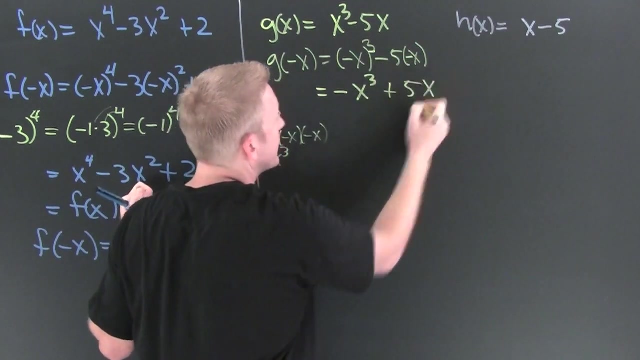 Why? Why, Because minus x mm-hm, minus x times minus, x times minus x. Okay, Minus and minus minus make minus x. to the third, which is what I wrote right there: Okay, Minus and minus make minus plus five x. 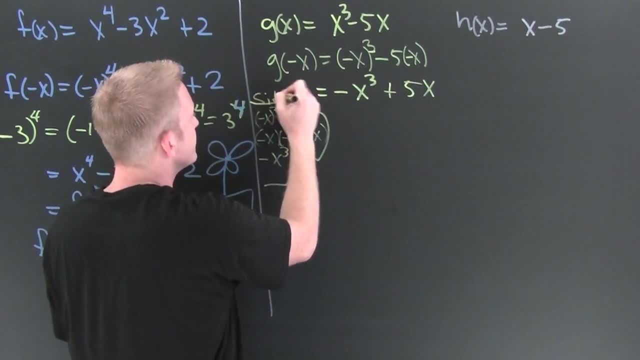 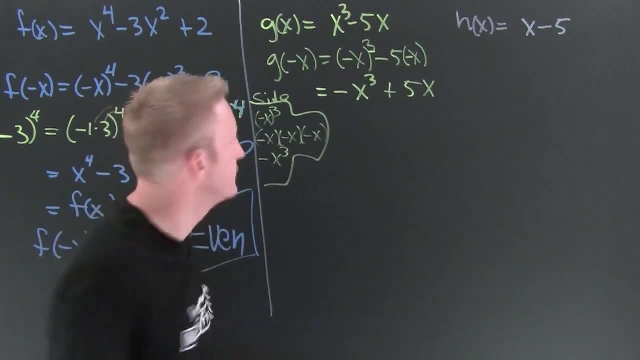 Mm-hm. Yes, Now, what do I want to do? I want to try to go and try to find the original function. Yes, In order to do that, what I am going to do is I'm going to pull out a little bit of this. 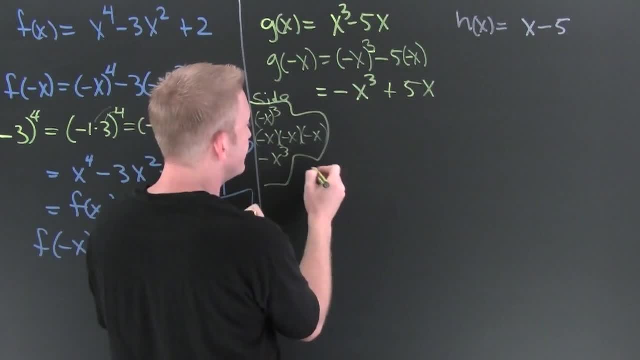 to do that. what I am gonna do is I'm gonna pull out a minus sign, mm-hmm, it's gonna pull out a minus and then, left over on the inside, I have X to the third minus 5x. but what is that? that's my original G of X. oh, so I have minus G. 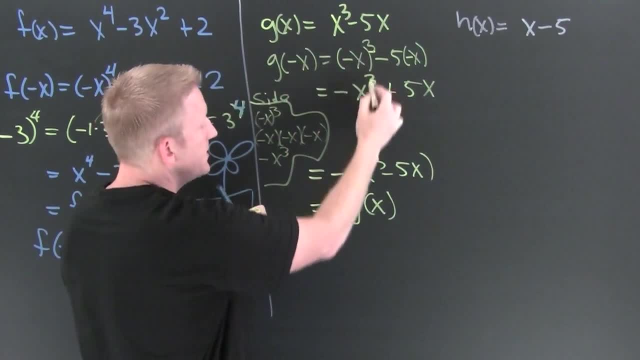 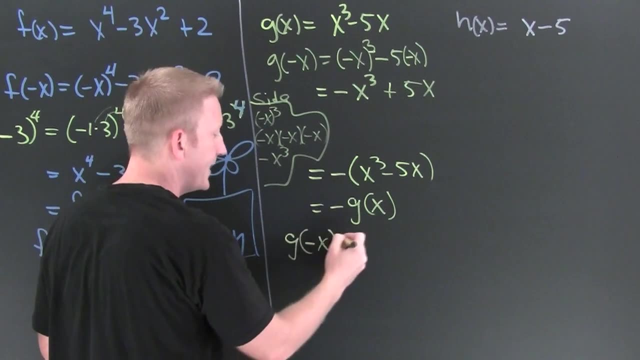 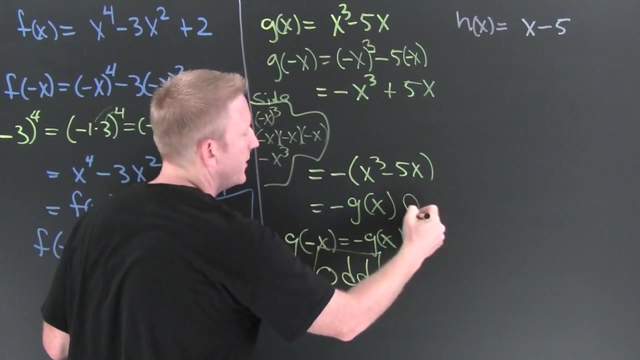 of X. so then it follows, G of minus X is gonna be minus G of X, and because G of minus X is equal to minus G of X, we can say that that that that one's a little off. um, so is he no? um, odd, yeah sure is one, two, three, four. I had to get that odd. 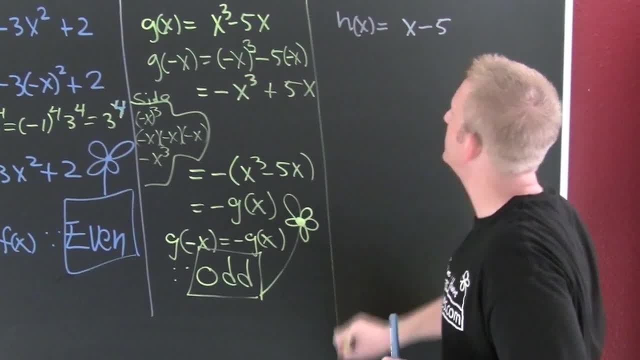 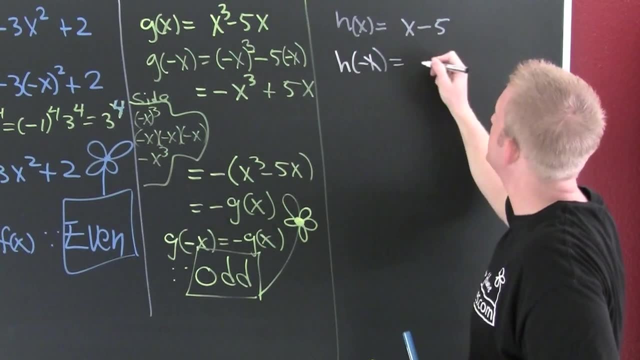 one in there. yes, now I'm up here. oh wait, I'm gonna try that same dang thing. mmm, I'm looking for H of minus X. yes, This is going to be minus X minus 5.. Oh boy, Maybe I want to try that same trick.